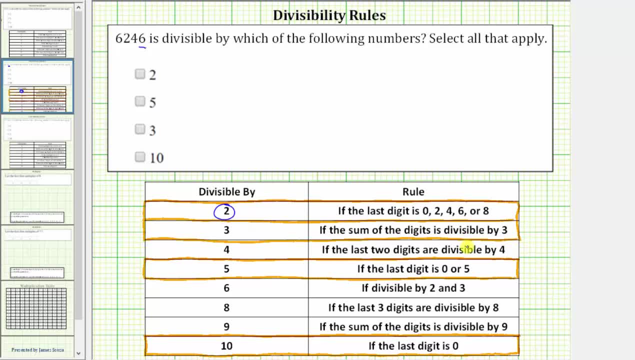 is divisible by 3.. So for this test, we must sum the digits of 6246, which would be 6 plus 2 plus 4 plus 6, which is equal to 18, because 18 is divisible by 3,. 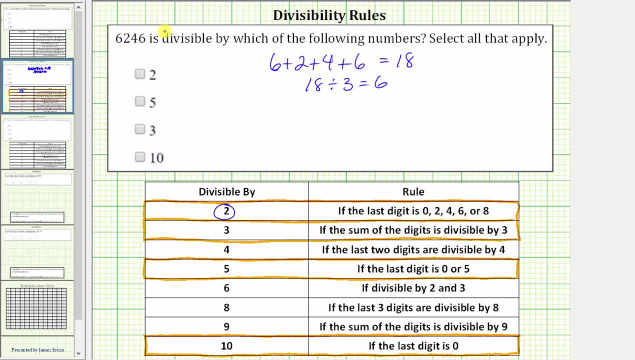 so is 6246.. Let's go ahead and circle 3.. Now we'll skip down to the divisibility rule for 5.. A number is divisible by 5 if the last digit is 0, or 5.. The last digit is 6 in 6246, and therefore the number is not. 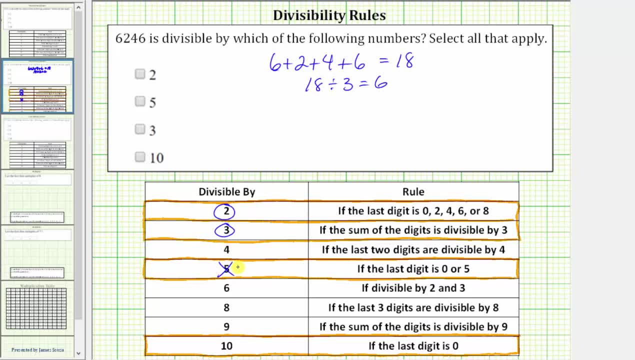 divisible by 5.. Let's go ahead and cross off 5.. We'll look at 10.. A number is divisible by 10 in 6246 and 7 in 6246,, which would be equal to 18,, which represents 60,, which means that there is no divisibility. 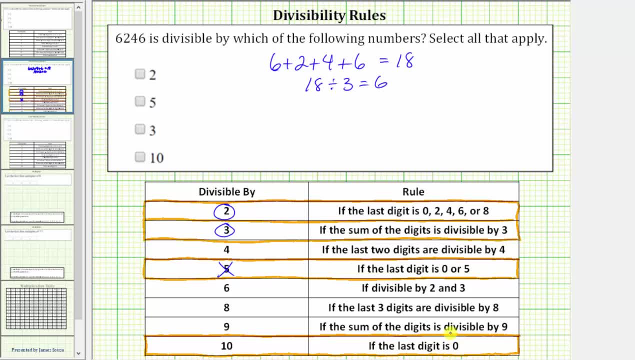 divisible by 10. if the last digit is zero, Again the last digit is six and therefore 6,246 is not divisible by 10.. If a number is not divisible by five, it will never be divisible by 10.. So to answer the given question, we select two and three. 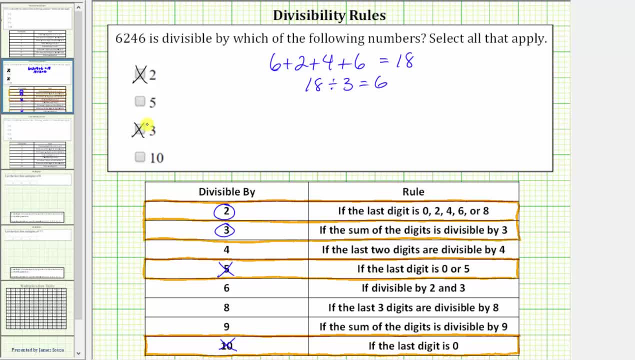 So, while we are done with this question, let's go through the divisibility test. for four, six, eight and nine as well, A number is divisible by four. if the last two digits are divisible by four, The last two digits of 6,246 is 46.. 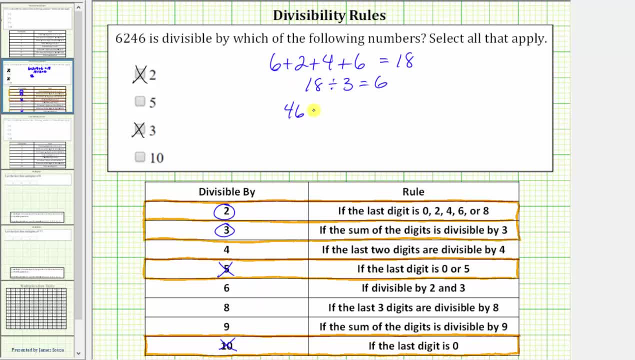 46 is not divisible by four, because if we try to divide by four, there will be a remainder, So we cross off four. A number is divisible by six if it's divisible by two and three. And notice how 6,246 is divisible by two and three. 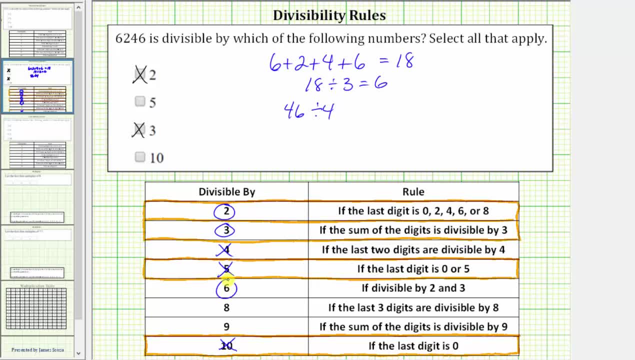 and therefore it's also divisible by six. A number is divisible by eight. if the last three digits are divisible by eight, The last three digits are 246.. 246 is not divisible by eight because if we divide, we will have a remainder.